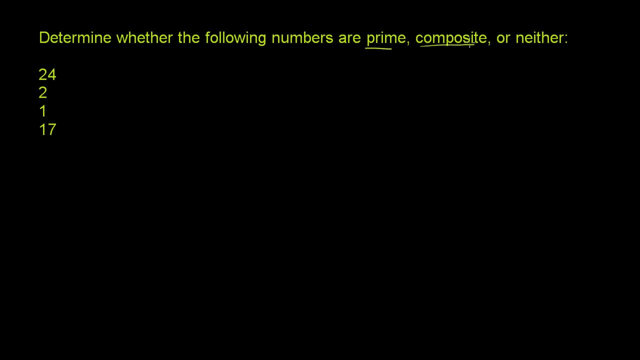 Determine whether the following numbers are prime, composite or neither. So, just as a bit of review, a prime number is a natural number, so one of the counting numbers 1,, 2,, 3,, 4,, 5, 6, so on and so forth. 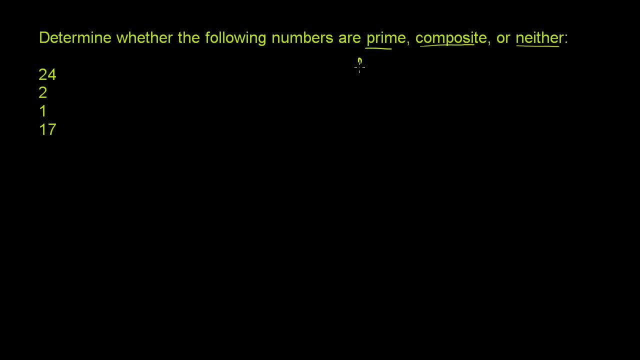 that has exactly two factors. So its factors are 1 and itself. So an example of a prime factor is 3.. There's only two natural numbers that are divisible into 3, 1 and 3.. Or another way to think about it is the only way. 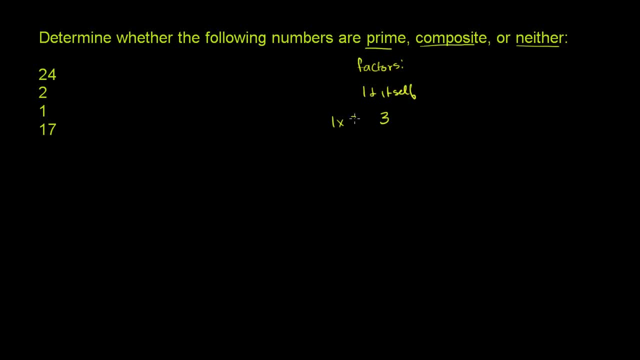 to get 3 as a product of other natural numbers is 1 times 3. So it only has 1 and itself. A composite number is a natural number that has more than just 1 and itself as factors, And we'll see examples of that. 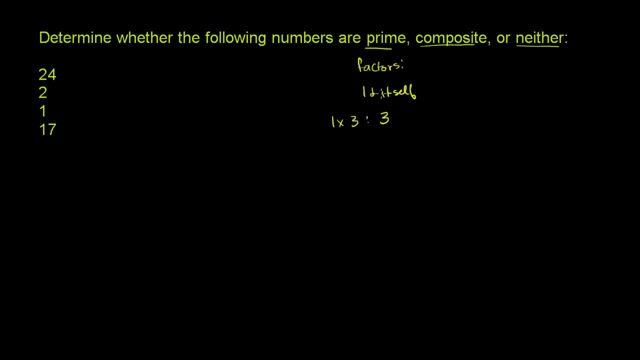 And neither will see an interesting case of that in this problem. So first let's think about 20.. So let's think about all of the. I guess you could think of it as the natural numbers or the whole numbers, although 0 is also included in whole numbers. 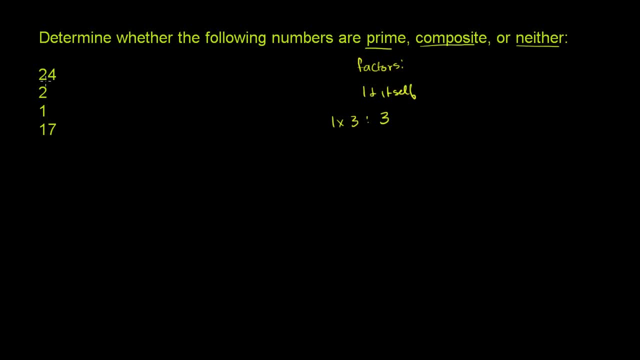 Let's think of all of the natural counting numbers that we can actually divide into 24 without having any remainder. We'd consider those the factors. Well clearly, it is divisible by 1 and 24.. In fact, 1 times 24 is equal to 24.. 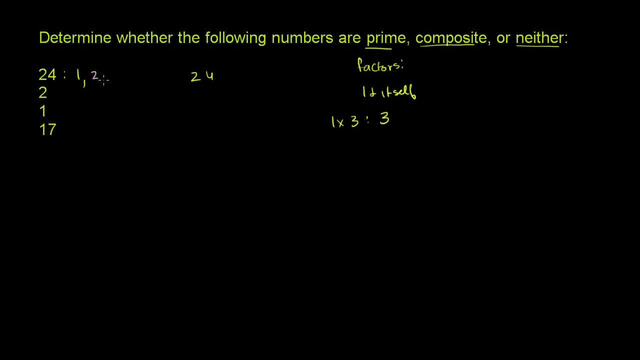 But it's also divisible by 2.. It's also divisible by 2.. 2 times 12.. 2 times 12 is 24.. So it's also divisible by 12.. And it is also divisible by 3.. 3 times 8 is also equal to 24.. 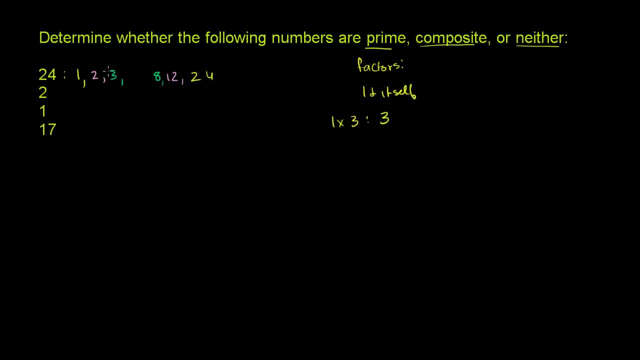 And even at this point we don't actually have to find all of the factors to realize that it's not prime. It clearly has more factors than just 1 and itself. So then it is clearly going to be composite. Now let's just finish factoring it, just since we started it. 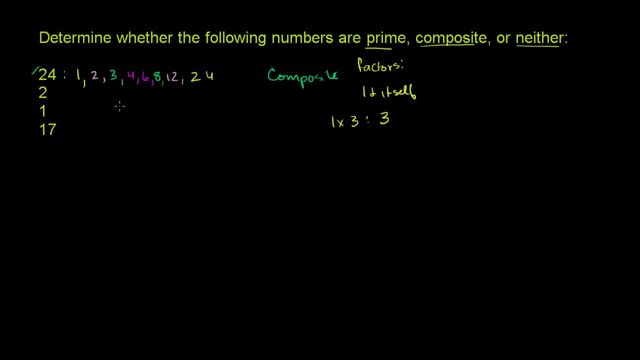 It's also divisible by 4. And 4 times 6 had just enough space to do that. 4 times 6 is also 24.. So these are all of the factors of 24, clearly more than just 1 and 24.. 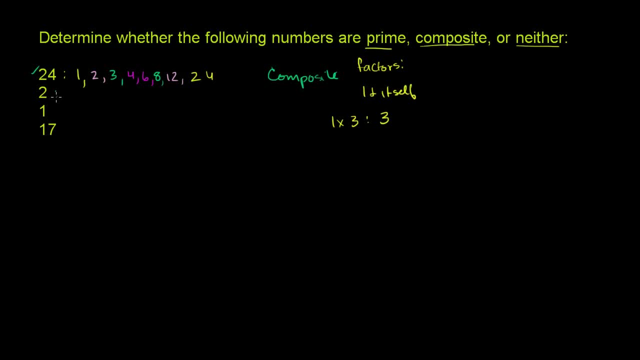 And now let's think about 2.. Well, the non-zero whole numbers that are divisible into 2, well, 1 times 2 definitely works 1 and 2.. But there really aren't any others that are divisible into 2.. 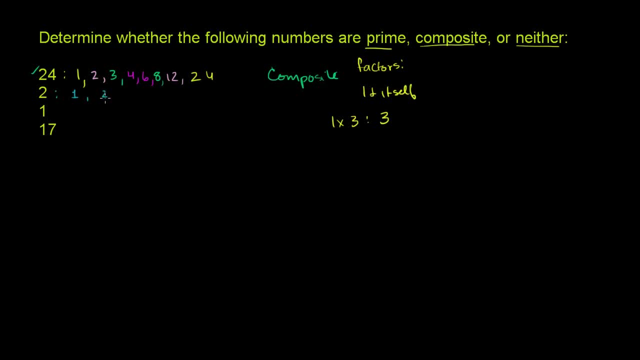 And so it only has two factors, 1 and itself, And that's the definition of a prime number. So 2 is prime And 2 is interesting because it is the only even prime number, And that might be common sense to you. 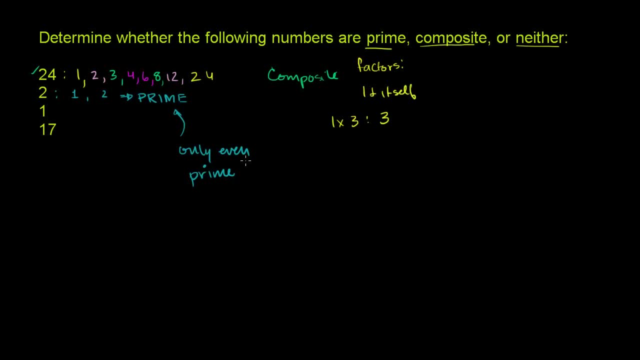 Because by definition, an even number is divisible by 2.. An even number is divisible by 2.. So 2 is clearly divisible by 2.. That's what makes it even, But it's only divisible by 2 and 1.. 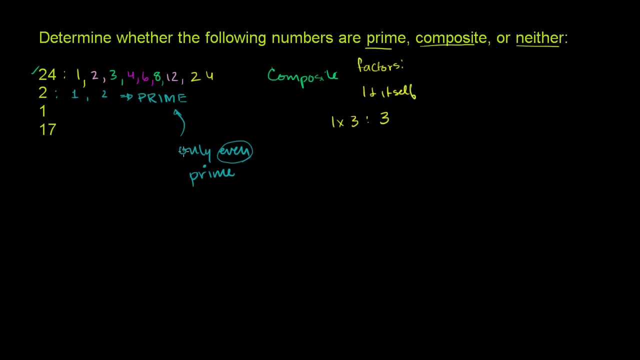 So that's what makes it prime. But anything else, that's even, is going to be divisible by 1, itself and 2.. Any other number that is even is going to be divisible by 1, itself and 2.. So by definition it's going to have 1 in itself. 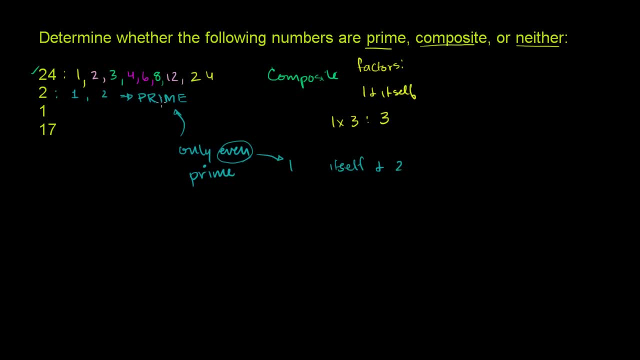 and something else. So it's going to be composite. So 2 is prime. Every other even number other than 2 is composite. Now here's an interesting case: 1.. 1 is only divisible by 1. So it is not prime technically. 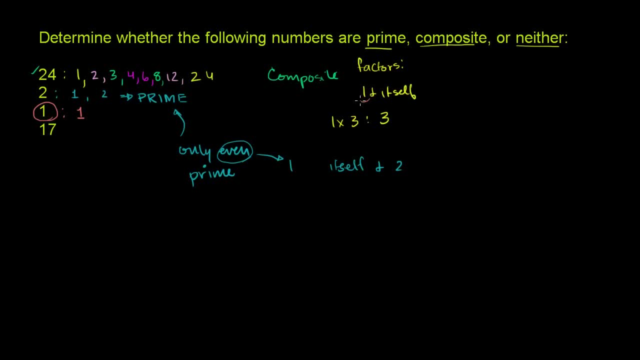 because it only has 1 as a factor. It does not have two factors. 1 is itself, But in order to be prime, you have to have exactly two factors. 1 has only 1.. It has only one factor. In order to be composite, you have: 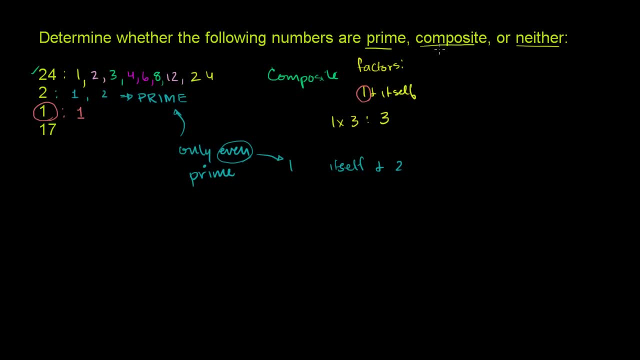 to have more than two factors. You have to have 1, yourself and some other things, So it's not composite. So 1 is neither prime nor composite, 1 is neither. And then finally, we get to 17.. 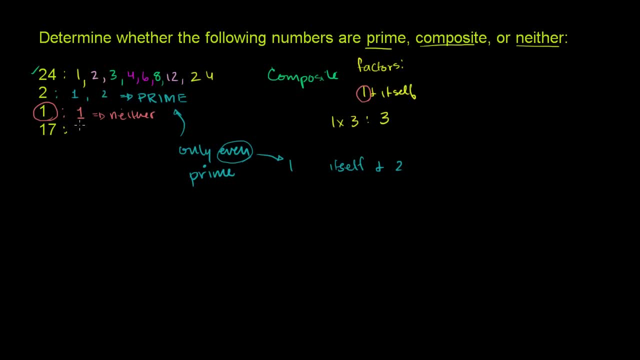 17 is divisible by 1 and 17.. It's not divisible by 2, not divisible by 3,, 4,, 5,, 6,, 7,, 8,, 9,, 10,, 11,, 12,, 13,, 14,, 15, or 16..